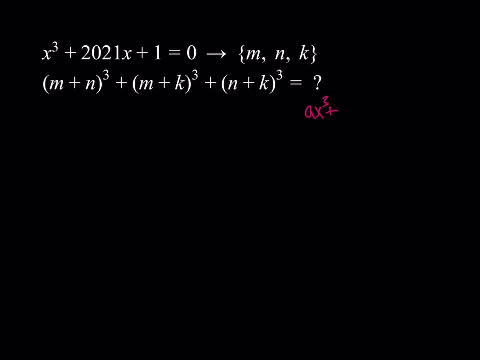 write your cubic as: ax, cubed plus bx, squared plus cx plus d is equal to zero. we have b equals zero. awesome. now what is that supposed to mean? well, you know that in a cubic equation, x1 plus x2 plus x3 is equal to negative b over a, which is always true for all any type of polynomial equation, right? 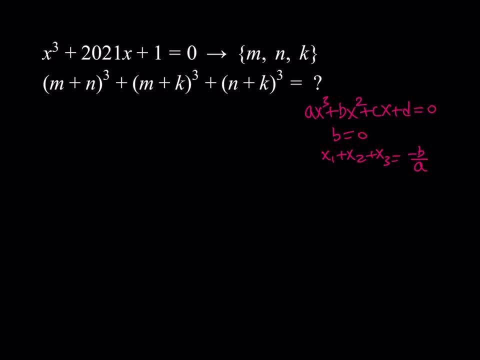 cubic, quartic, quintic doesn't matter. so if b equals zero, that means the sum of the roots is also zero. so from here we get the importance. conclusion: m plus n plus k is equal to zero. so that's, that's going to be our first relationship. 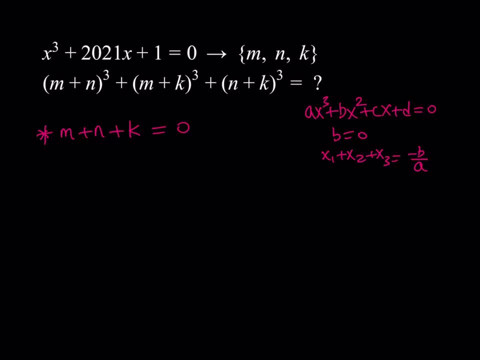 great, great. so, uh, what is my second one? well, second one is going to be the two-way products: mn plus mk plus nk. now, how do you find that? that's c over a, and in this case, c is the coefficient of x, but it's not c over a, it is actually c over a. i mean, what am i talking about? it's positive c over. 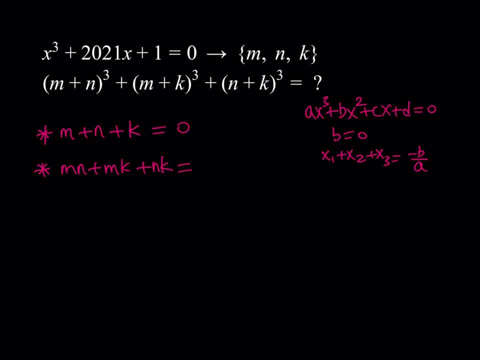 a. so it kind of goes like negative, positive, negative. they're going to alternate. so this is c over a and since a is one, this is just going to be 2021. cool, okay, nice. what else do i know? well, uh, the product which is going to be negative: d over a. 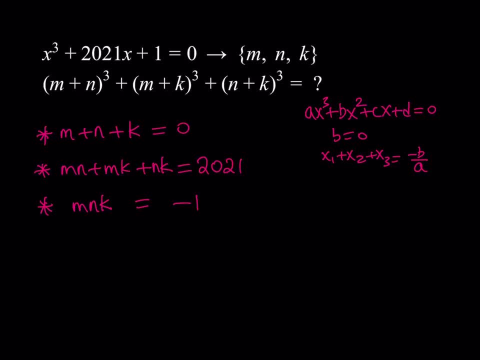 in this case, is going to be negative one. cool, you can again look at that video for reference for vieta's formulas. now, uh, what am i going to do with this? well, i'm supposed to evaluate this expression and i'm going to use- i'm going to be using- these. 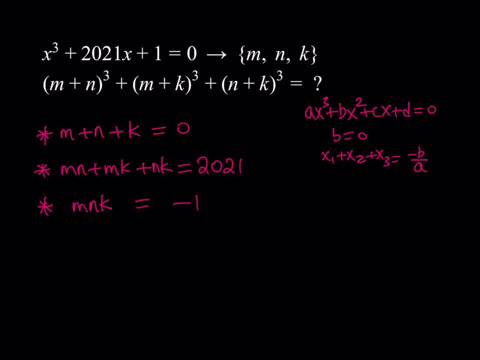 like i said earlier, i'm going to present two methods. here's the first solution method. first of all, notice that these expressions m plus n, m plus k and n plus k without the cubes give us something interesting. if you add them, what do you get? without the cubes, of course. 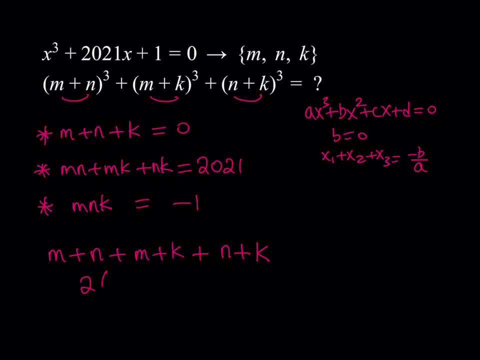 if you add them without the cubes, you get two times m plus n plus k, right? well, we know that m plus n plus k is equal to zero. so this is also zero, because two times zero equals zero, right? what is that supposed to mean? if you add them without the cubes, you get two times m plus n plus. 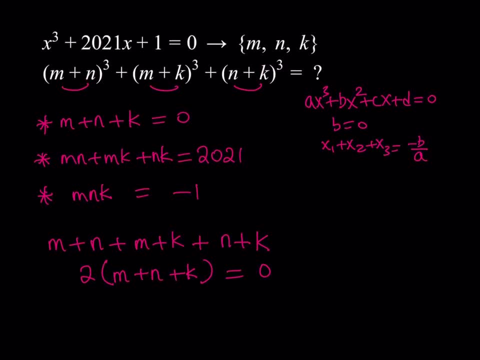 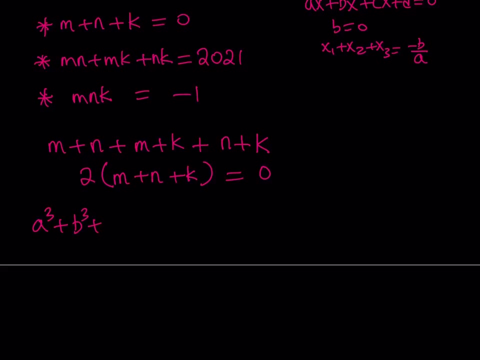 k. what does that mean? well, it is significant because we have a special expression for that. if a plus b plus c is equal to zero, then a cube plus b cube. okay, what am i talking about? okay, let me write it down. let me write it down. here's the formula. in other words, we can subtract this: 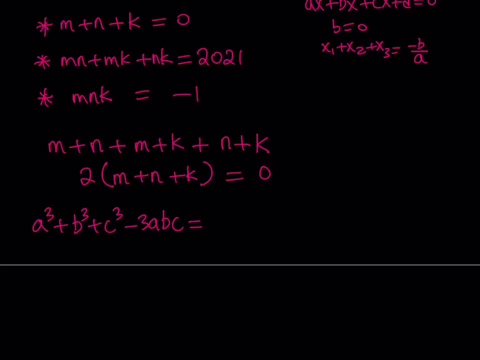 weird polynomial. and to make matters worse, this polynomial is divisible by a plus b plus c. would you believe that? well, if you don't, you can kind of verify it. but yes, it is. so this polynomial is divisible by a plus b plus c and the other factor. and again, we've done this in. 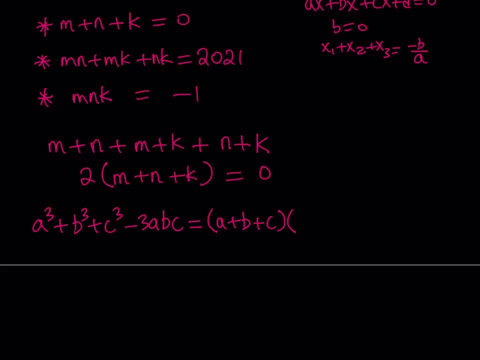 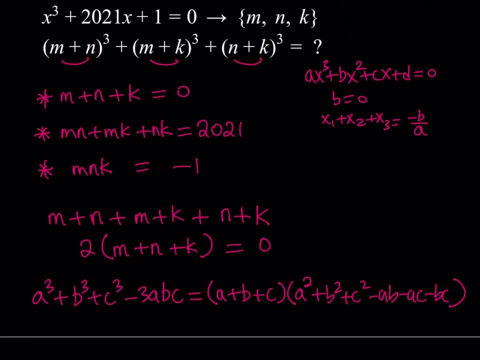 another video, so you can also look at that too. maybe i'll try to include that link as well. and the other factor is going to be a squared plus b, squared plus c, squared minus ab, minus ac, minus bc. now why is this significant? it is significant because if you call this a, if you call this b, 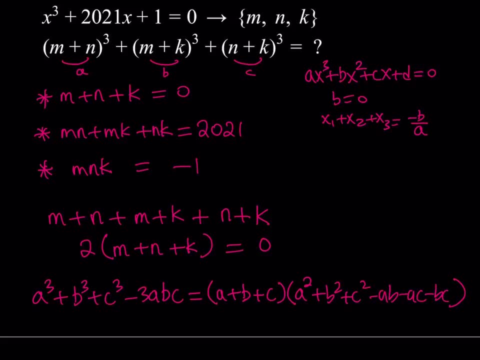 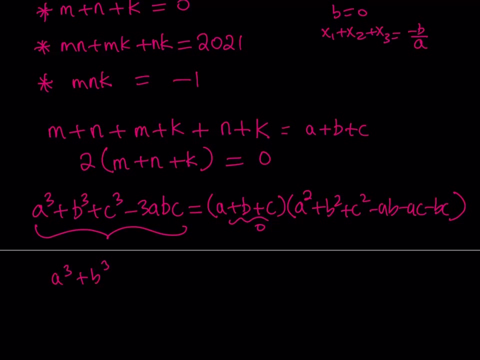 and if you call this c, we have that a plus b plus c is equal to zero. this is a plus b plus c, right? well, if a plus b plus c is zero, that means this is zero. therefore, this is also going to be zero, which means you have a cube plus b, cube plus c, cubed being equal to 3abc. 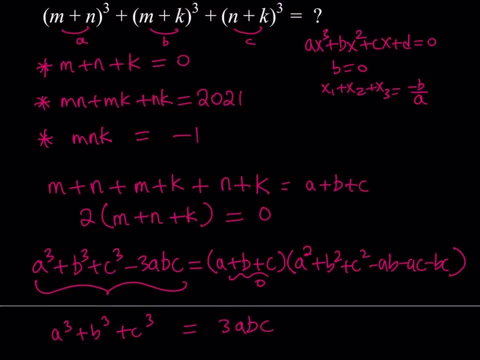 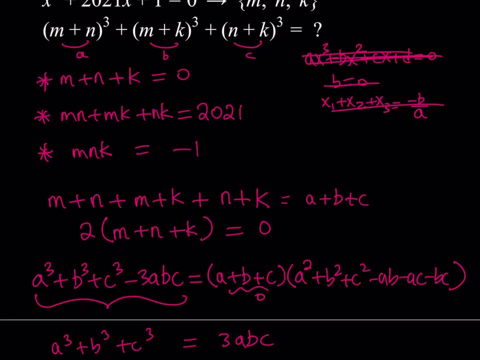 nice. so what am i trying to find? well, i'm trying to find a cube plus b cube plus c cubed. that's what i'm trying to find. well, by the way, this, this a and that a are different things, so don't worry. well, what is abc? well, abc is not the m and k, of course. it is the product of all these quantities. 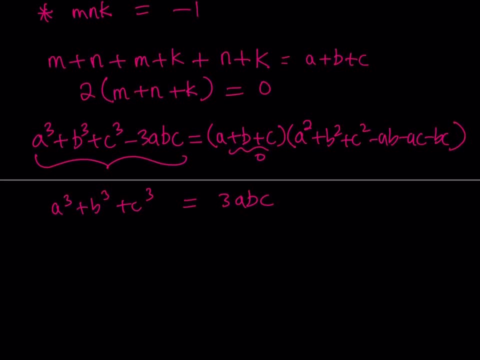 without the cubes. so i'm trying to solve for this. and so, in other words, m plus n cubed plus m plus k cubed plus n plus k cubed is equal to three times m plus n times m plus k, times n plus k. now you might be asking, like, what is so significant about if you're trying to find? 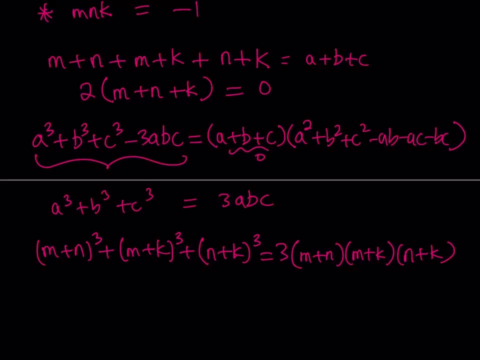 this, but now you complicated things. do we know how to find this? well, you can go ahead and distribute, and obviously this is better than the other one, because that's a sum of cubes. this is kind of like a product, a lot easier to handle. but again, we're gonna make it nicer. this is not nice enough and 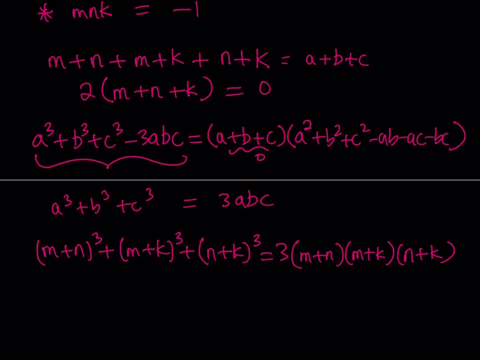 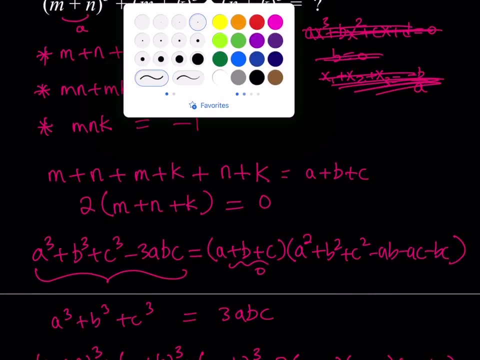 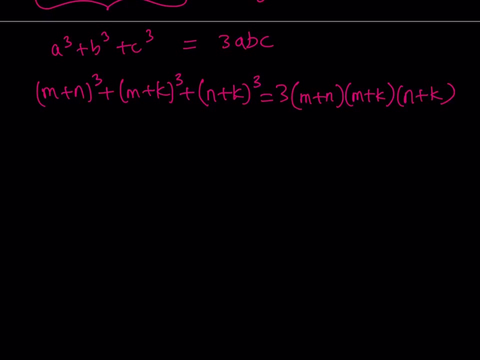 i'm going to make it nicer how we're going to use the relationship again and it up keeps popping up. so it's a super important relationship that m plus n plus k is equal to zero. this is super duper important. why? because if you look at this, if i know that m plus n plus k is equal to zero. 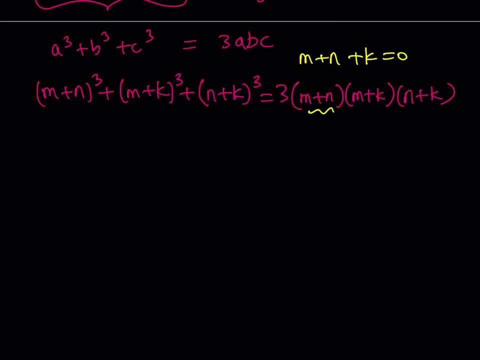 that allows me to write each one of these in terms of the third one, for example, m plus n can be written as negative k, m plus k can be written as negative n and plus k can be written, so what is that supposed to mean? what i'm trying to find, then, is equal to negative, because i'm 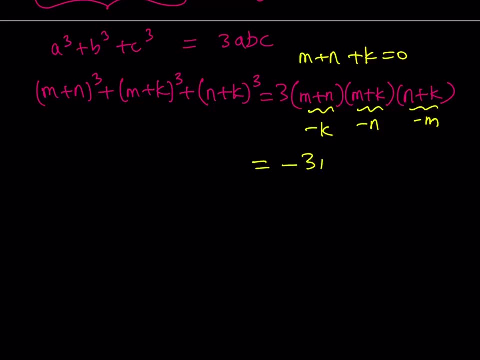 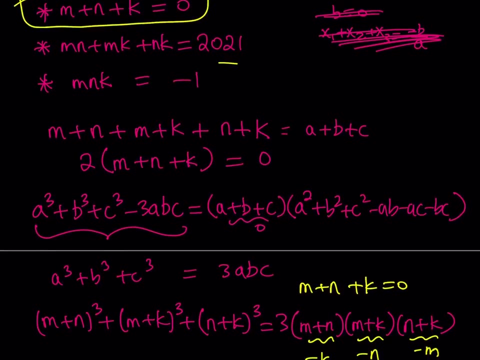 multiplying three negatives, that makes a negative negative three: m and k. well, do i know m and k? yes, i do remember. at the beginning we calculated it, so we do have that relationship and i told you that we were going to use it. now we're using it. m and k is equal to negative one from yata's. 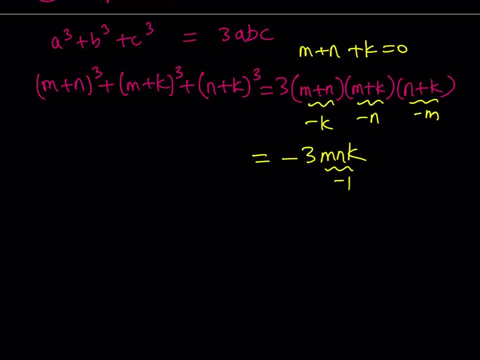 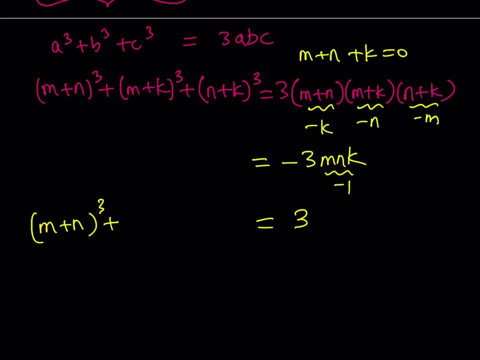 formulas: if this is negative, one negative, three times negative. one is positive, three. so what i was looking for, the expression, this gigantic expression here: the sum of three cubes is equal to three. that concludes the first solution method. okay, so the answer is three. now i'm going to present 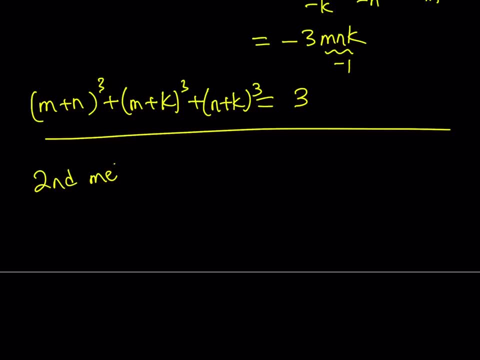 the second method, and then you can decide. please let me know in the comment section which method you think is better or which method you like better. of course, everybody has their own preferences and i will also share mine. okay, second method involves a little different strategy. well, i can't say completely different, but let's start with what we're trying. 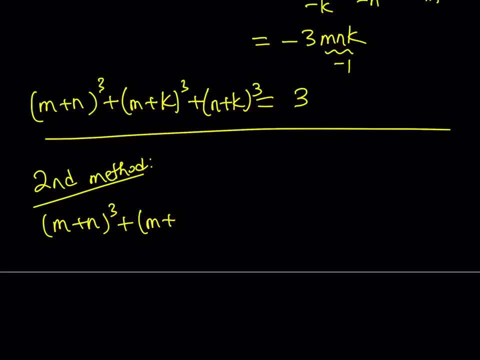 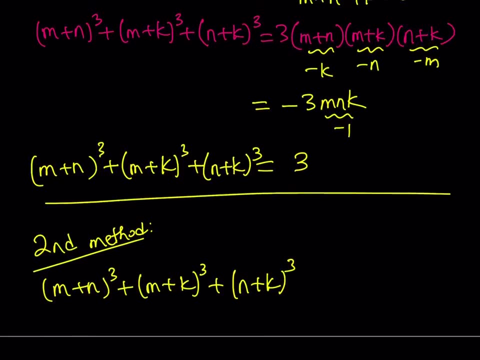 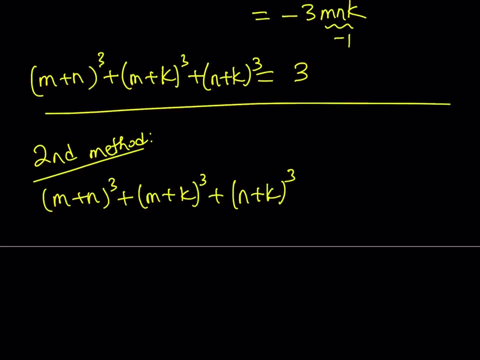 to find this one, okay, so i'm trying to simplify this or find the answer again. we're gonna go back to this idea here. m- we're using it at the beginning, in other words: right, it's kind of easier, i don't know. m plus n is equal to negative k. this is equal to negative n, so let's go ahead and write that. 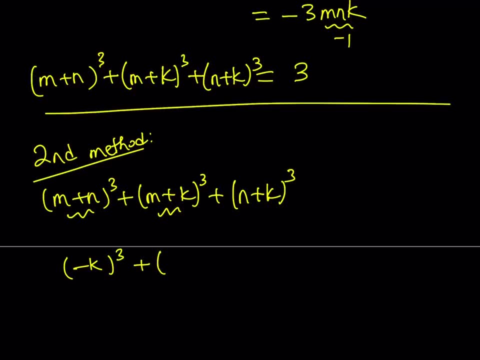 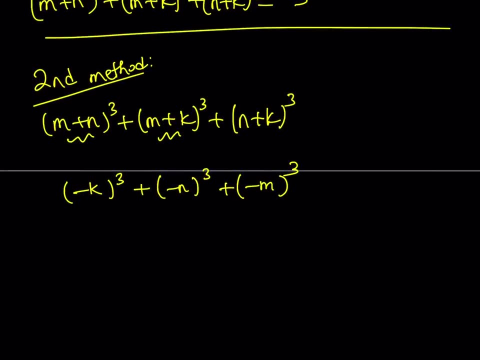 negative k cubed plus negative n cubed, plus negative m cubed. great, now if you keep a negative number, you get a negative answer. so they're all going to be like negative k cubed, negative n cubed, negative m cubed, and obviously we can put a. 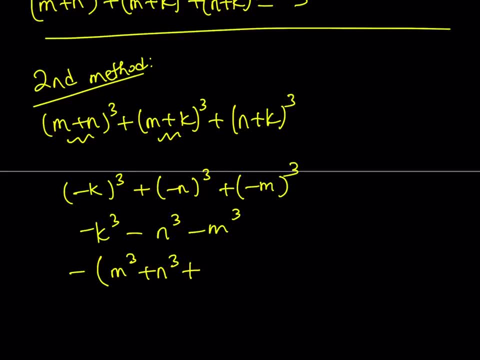 negative sign on the outside and write them in kind of alphabetical orderish right, something like this. and you're going to get that. so what i'm trying to find is actually equivalent to this. this is nicer because, um, it's not like a two-way, um addition cubed, it's just a singles cubed sort. 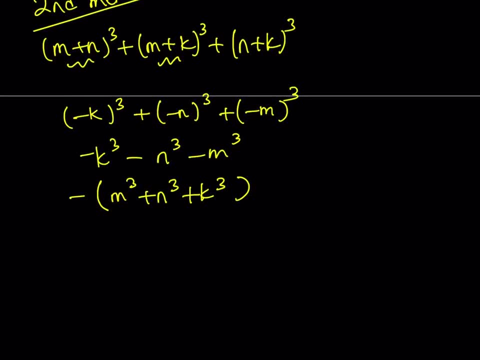 so this one is a little easier to find, but in order to be able to find that, i'm going to use a little algebra, which is kind of fun. i mean, the second method is going to take longer, but, um, it's a. there's a different flavor to it. okay, cool, let's take a look now. what am i going to do in order to 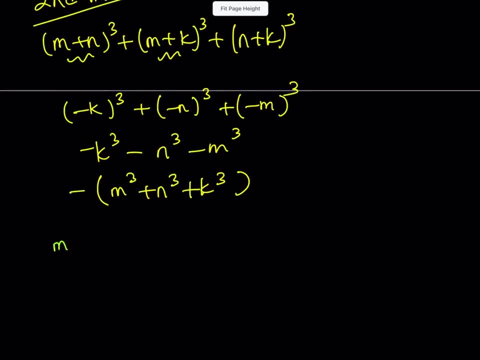 be able to get the sum of the two cubes, obviously, and i think that should be kind of obvious. i'm going to go ahead because we don't have a formula. okay, so we have a formula for a cube plus b cubed, but we don't have necessarily have a formula. well, 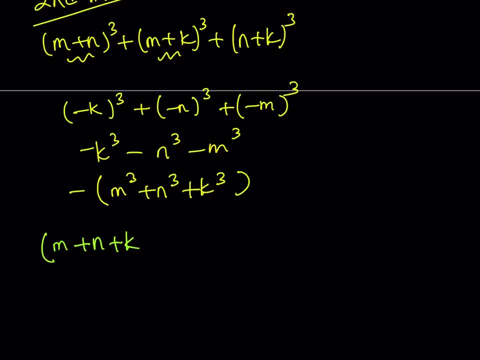 we kind of do. but whatever, let's just do it. okay, this is what i was trying to do. let's cube this expression. okay, what do you get when you cube it? well, i can treat this as a single identity or single entity, whatever, or single expression, and then do it that way, kind of like a plus k. 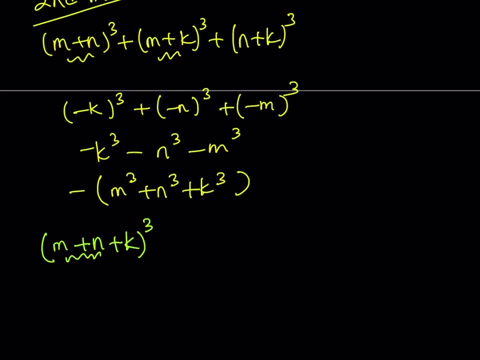 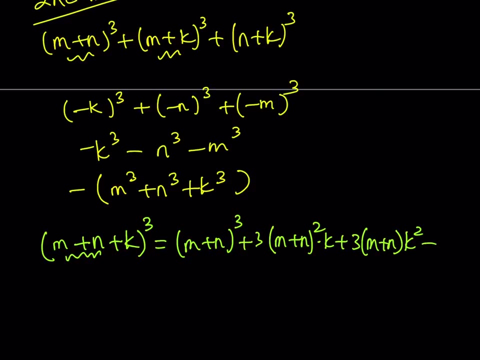 cubed, or z plus k cubed, that makes sense. okay, it's going to look like this: m plus n is going to be my first term. cubed plus three, again using the binomial theorem. i'm just gonna, you know, write up, okay, like this, and then finally, k cubed. cool, of course this requires a little bit of expansion. 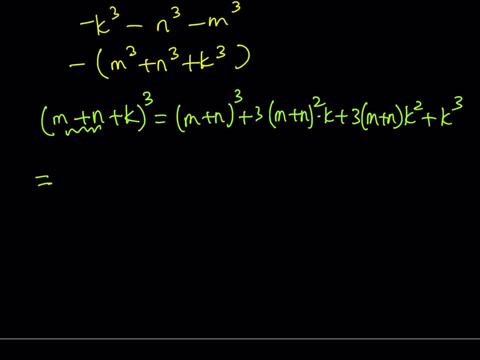 here, and if you do expand it, uh, you're gonna get something nice. well, it's not gonna be super nice, but i can't guarantee that right. 3m squared n plus 3m n squared, i'm probably gonna need a little more space. i feel like let me start over here all the way here, so kind of like, uh, let's see. 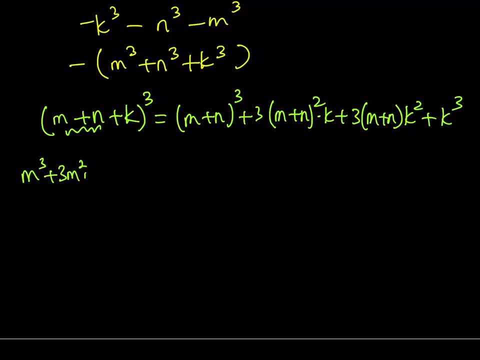 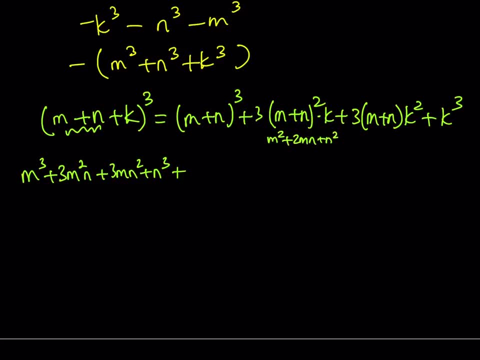 plus 2mn plus n squared, and you're going to multiply it by 3k. so consider that it's going to look like 3k m squared plus 6mn k. kind of looks like square kilometers, right, okay, and then multiply 3k by that you're going to get 3k n squared. when you distribute that you're going 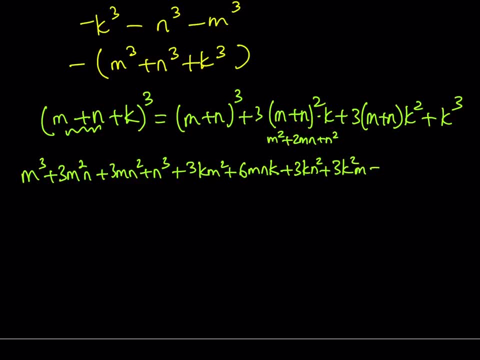 to get 3k squared m, 3k squared m plus 3k squared n, and then, finally, you're going to be getting k cubed. okay, that's kind of like a mouthful right, but we're going to arrange these terms and, trust me, it's going to simplify, it's. 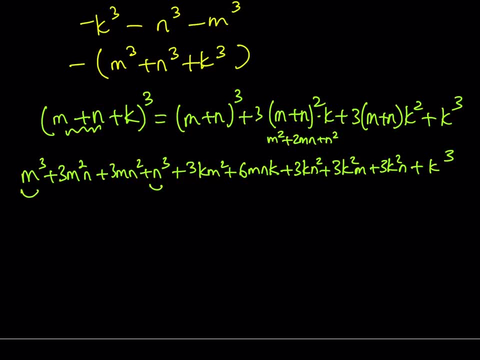 going to be really nice. i'll take m cubed plus n cubed plus k cubed, because that's what i'm trying to find- remember our expression depends on this- but just the negative of it. so once i find the answer from here- m cubed plus n cubed plus k cubed- i'm just going to negate it. that's going to be. 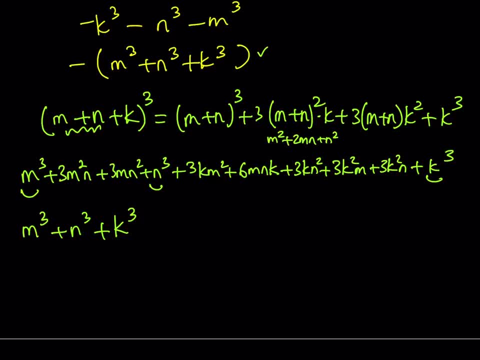 the answer. cool, so that's the first part. the second part is going to be the answer to the second part. i gotta be smart and put these together in a meaningful way. how well, i gotta take these two together, but factor out 3mn and write it like this, because you'll see in a little. 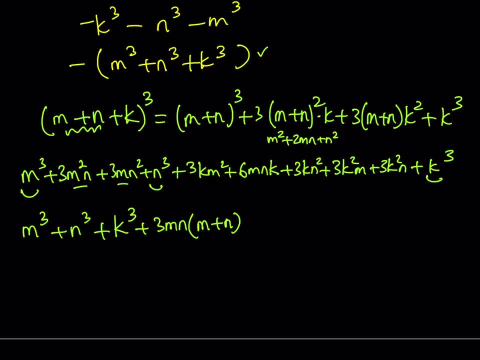 bit okay. and then the next thing you're going to look at should be something like these two, because again they're kind of friends, good friends, whatever. 3km times m plus k, you get the idea these two guys are going to go next and then that's going to be 3kn multiplied by k plus n. 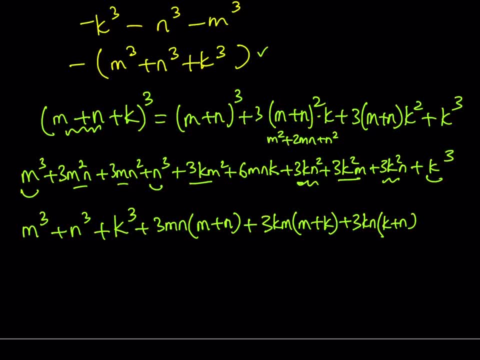 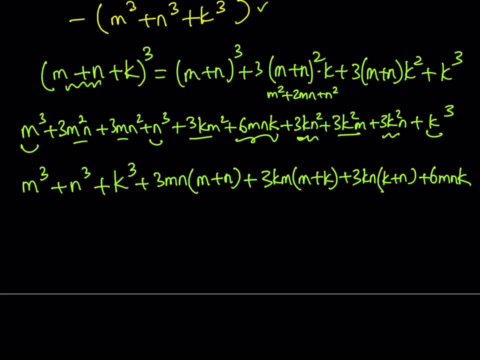 you get the pattern hopefully, but we still have a leftover, and that is the, the glorious term, which is 6mnk. it's kind of like by itself, right? so this is basically a formula kind of for m plus n plus k cubed, all right, but i'm trying to find the sum of the cubes. well, how does this help me? again, we're 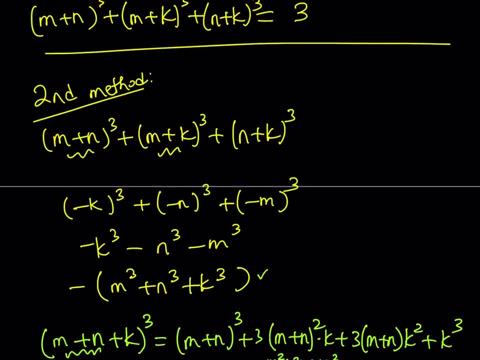 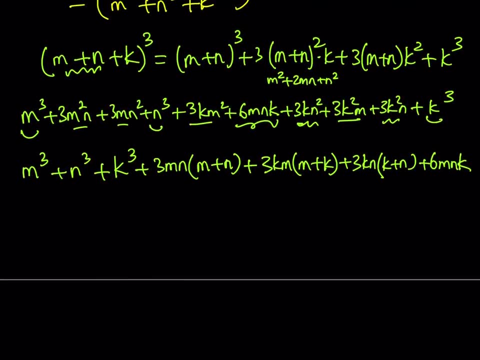 going to do the same idea. since m plus n plus k is equal to zero, m plus n can be written just like here: negative k and so on and so forth. right, so i can replace- i can replace m plus n with negative k. i can replace this with negative n, i can replace this with negative m. beautiful, awesome and you're. 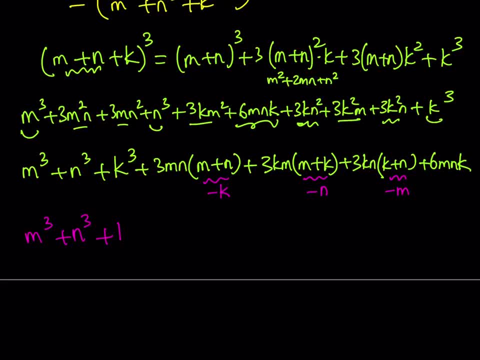 gonna see in a little bit why this is so awesome. because it's awesome, okay, cool. this is going to give me negative 3mnk, 3mnk minus 3mnk. you see how awesome that is. plus 3, i mean plus 6mnk. now notice that these two guys. 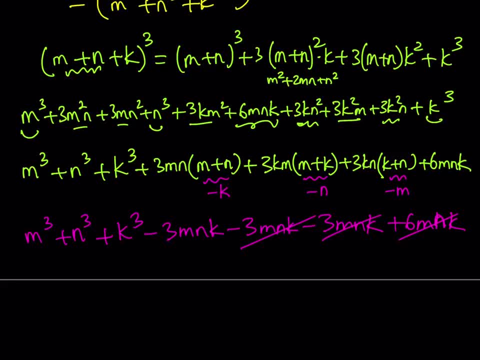 will cancel this out. we're going to end up with this guy over here. wow, that's interesting, but what was this whole thing equal to right? well, i was trying to expand this right? oh, this is where it comes from nice, but m plus n plus k is equal to zero. so this is equal to zero, wow. 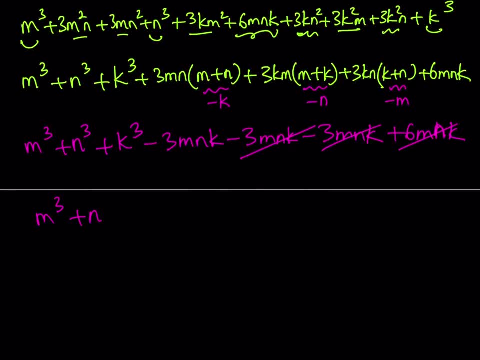 that's interesting, and i was trying to find something like this right. so in other words, in other words, this guy is equal to zero because it's equal to m plus n plus k, quantity cubed. well, what is that supposed to mean? if you isolate this sum, then it's going to equal 3mnk. 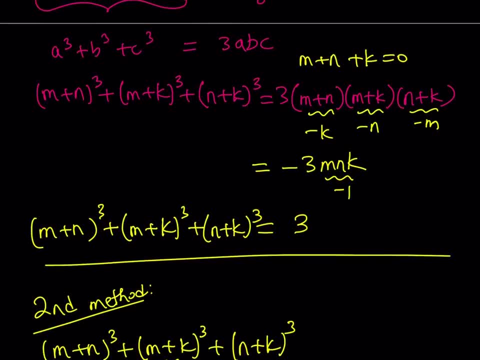 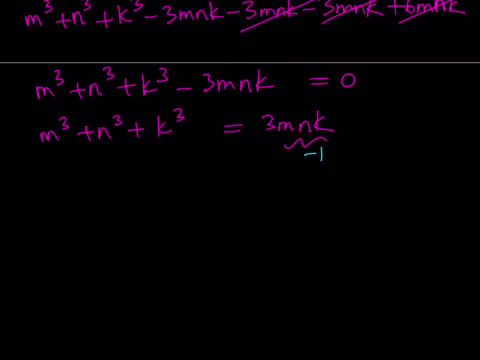 and we know that mnk is equal to. we found it before, right, didn't we? it's equal to negative one. awesome, so this is equal to negative one. what is that supposed to mean? well, if this is negative one, then this is equal to negative three. but if you remember, if you remember, m plus n cubed plus.